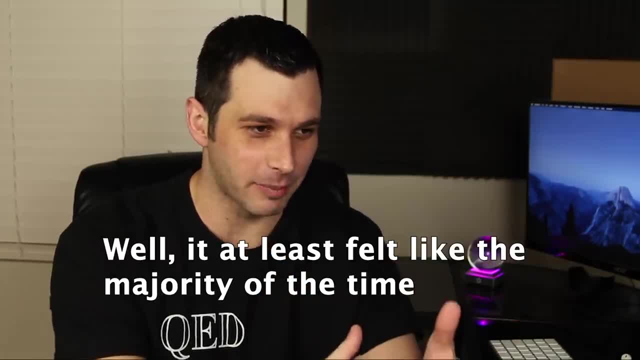 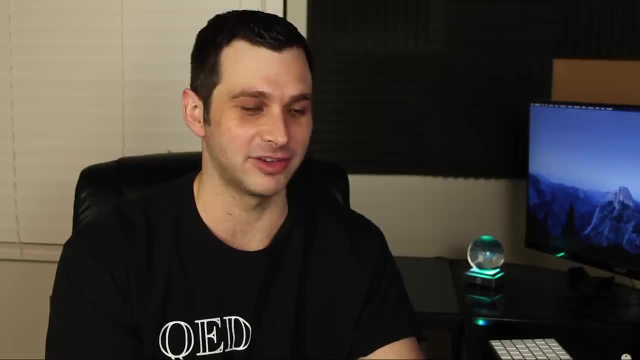 I want to say kind of the majority of the time staring at a problem and having no clue how to start it. And it wasn't like in any other class of staring at a problem and having no clue what to do, Because often I could try something, you know, whether it be moving x to the other side of. 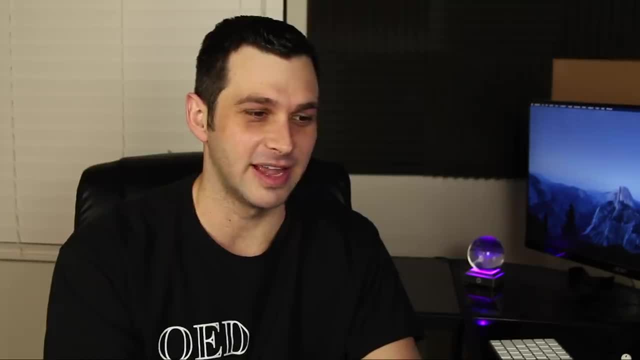 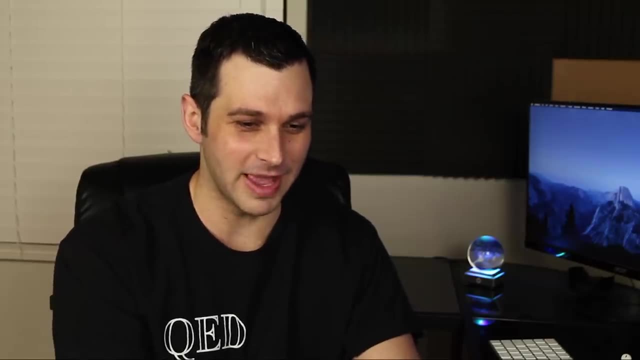 the equation, see if I can solve it, whatever it may be. Not in this case. Sometimes I could draw a picture, which is a good strategy, but it was often like staring blank page, no clue what to do, And sometimes I would figure it out after an hour and a half or whatever. 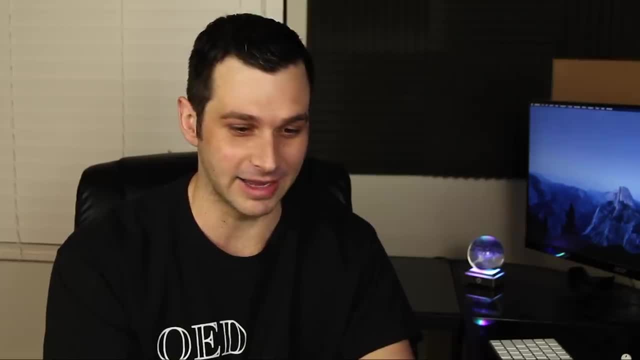 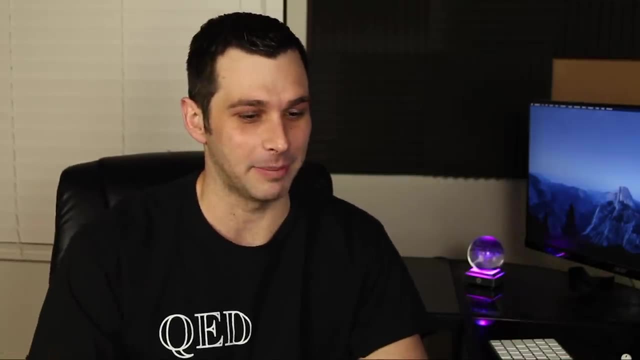 I'd be like, oh my god, this is what I have to do, And sometimes I had to give up, or else I would take three years going through this book. I don't recommend giving up, but realistically, it's going to happen. 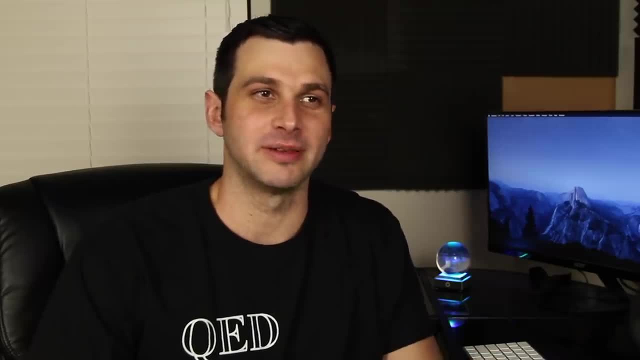 And in the next video I'm going to go through a proof from this textbook that should show you exactly what I'm talking about. It's a good proof, too, because pretty much anyone watching should be able to understand it, Even if you're in like Algebra 2, you should be totally fine. 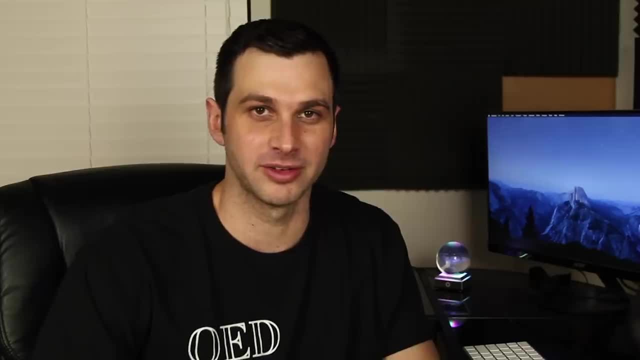 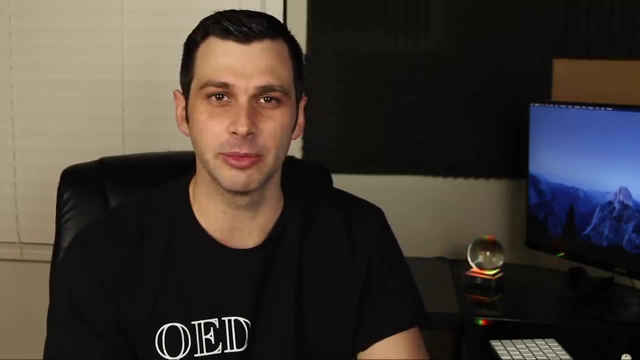 But I'll do that in the next one, so this video doesn't go on for like 30 minutes. Okay, so what is real analysis? for people who don't know, It is calculus 1 and 2, single variable calculus done rigorously. 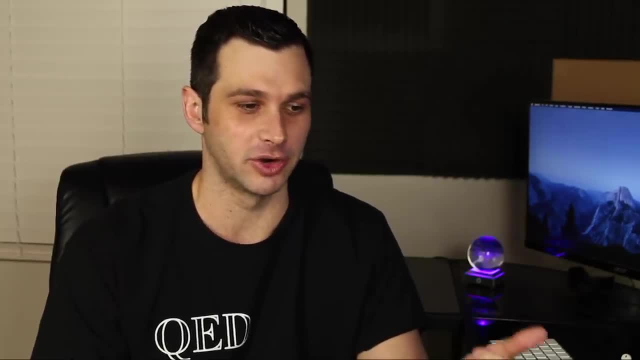 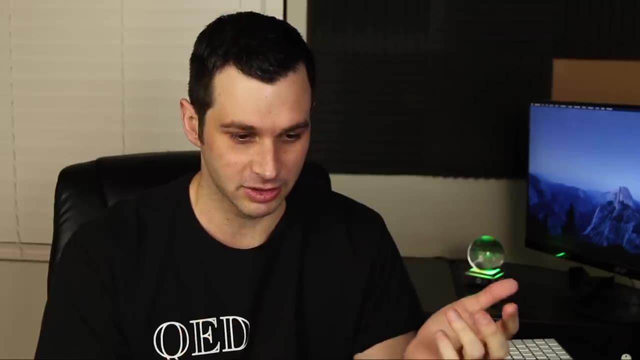 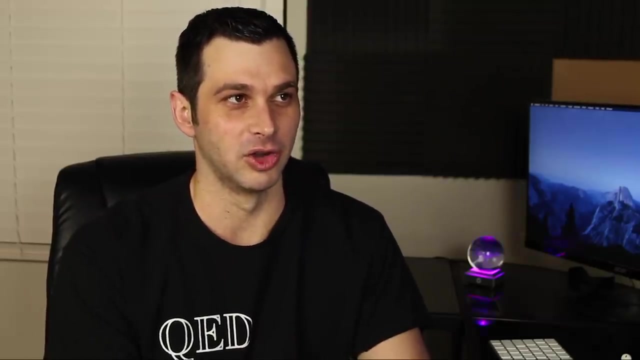 That's a good and bad definition. It's good because it's true. You learn limits, derivatives, integrals, sequences, series, Calculations, Continuity, differentiability, convergence, divergence, all that stuff rigorously. You learn it foundationally from the ground up. 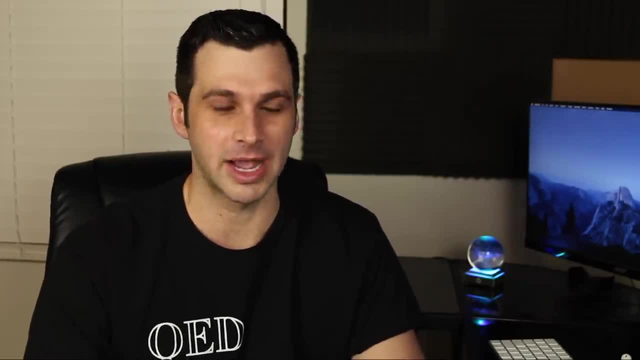 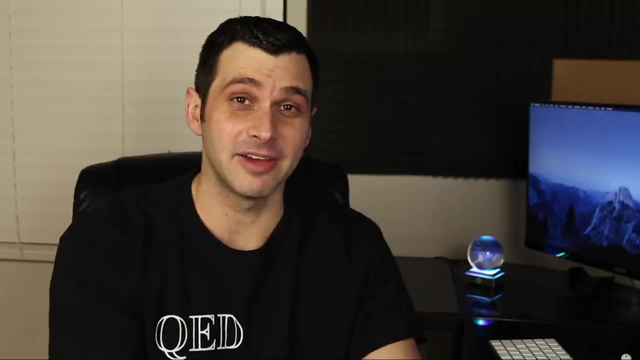 And there are a few other concepts you go into that you don't learn in Calc 1 or 2, like metric spaces or Fourier analysis. But for the most part that's what it is. But that's also a bad definition because in a way, because when you hear that you 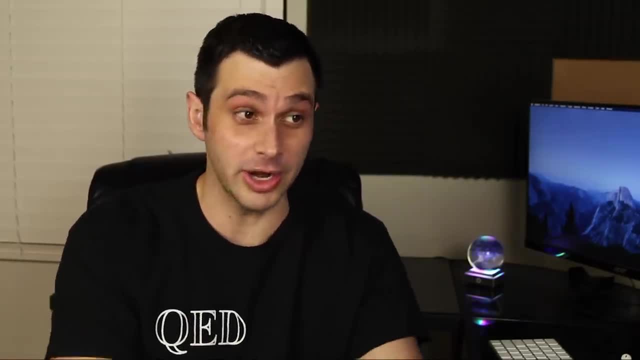 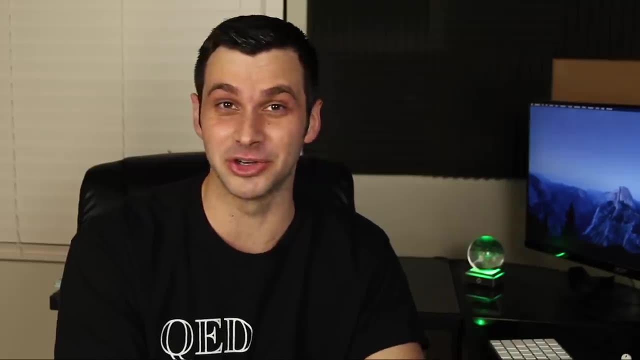 might think: oh, if you were good at Calc 1. You'd be good at real analysis. Or if you like Calc 1, you would like real analysis. Not the case. Not necessarily, It could be true, But not the case. 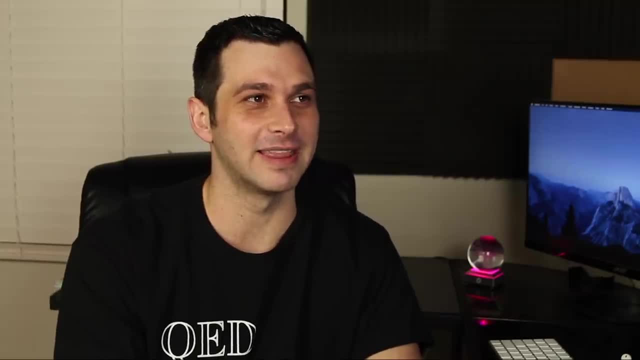 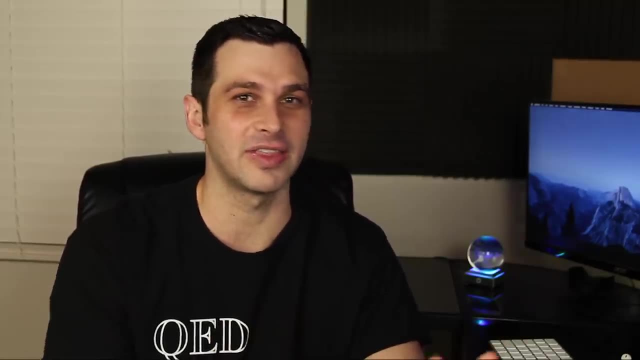 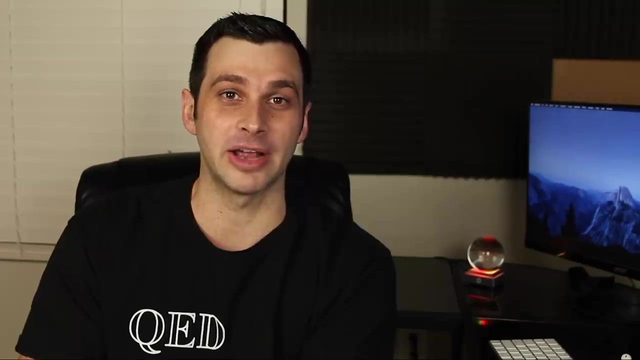 It is a totally different animal. In a pure math class like this you're not doing related rates, velocity and acceleration problems, optimization, nothing like that. You're doing stuff like find a function that's continuous at all the rational numbers but discontinuous at the irrationals. 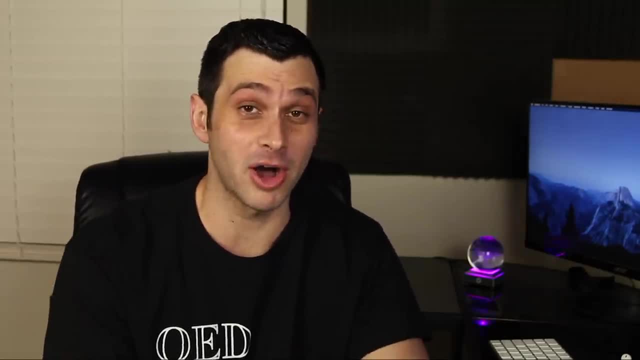 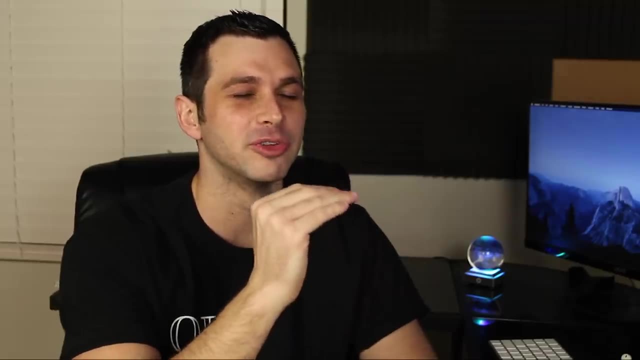 Or vice versa, Or prove that one of those is in fact impossible, And that is true. One of those is impossible And there was a chapter that you built up to that proof. It was the longest buildup ever to prove one of those is actually impossible. 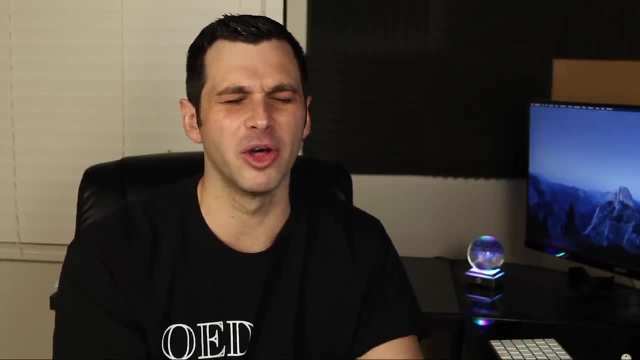 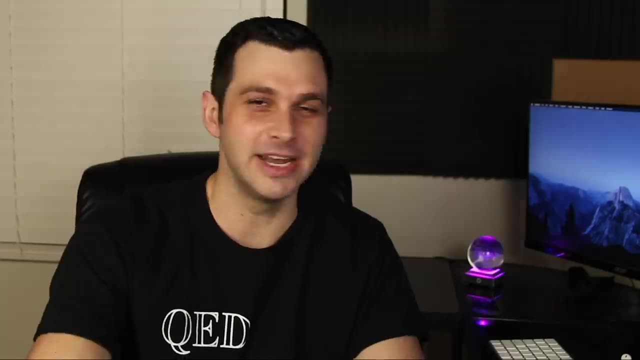 So you're doing stuff like that. It's not very applied, Although there are applications here, And what I mean by that is, you might be thinking, why would I ever need to know a function that's continuous at the rationals and not at the irrationals, or vice versa? 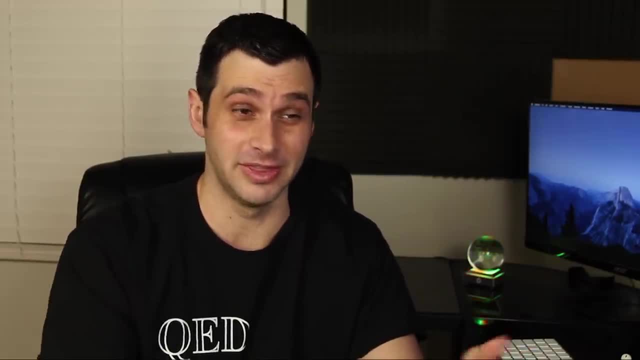 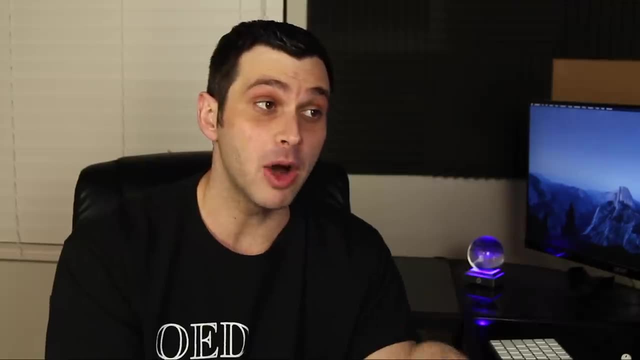 And you wouldn't- At least as far as I know- In a physical world or in a physics application. you wouldn't have to do that as far as I know. But once you're able to do a problem like that, or do a proof like that, you really understand. 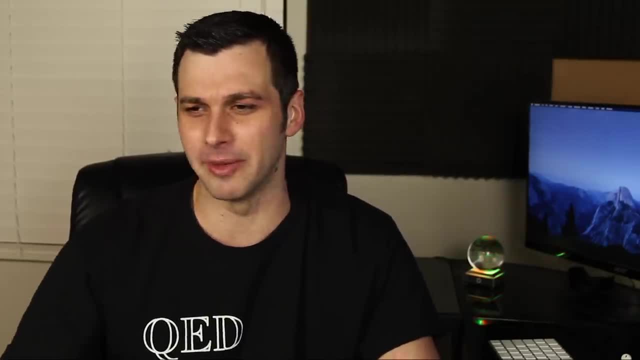 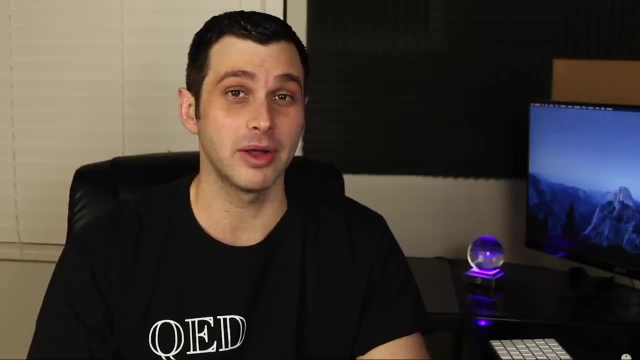 continuity much better than you did in Calc 1, where really the best answer you have is there are no holes or asymptotes or breaks in the graph. That's really all you got. Once you understand it well enough to answer questions like that. then, when you go on to 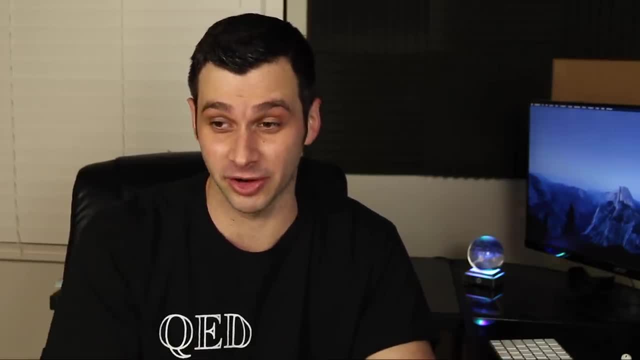 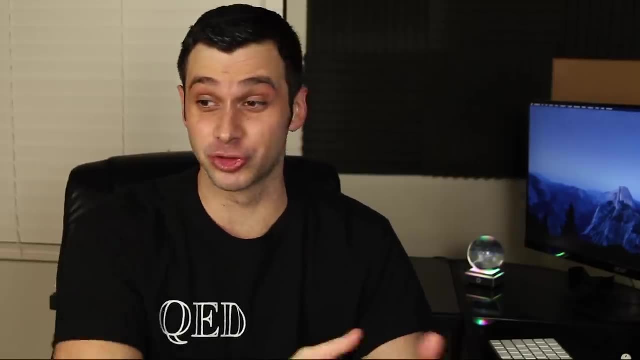 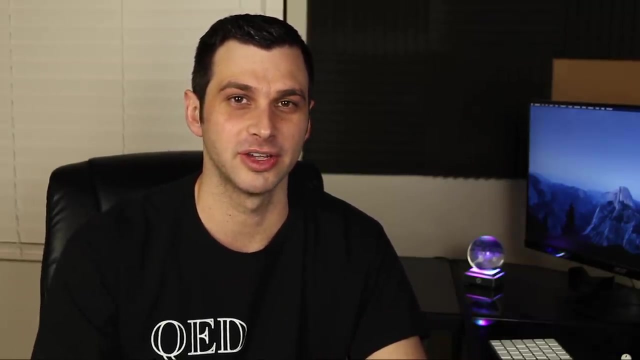 physical spaces and a continuous mapping from one space to another, which is a more generalized definition than a continuous function. you learn in real analysis. then you have the tools to rigorously understand that, And topology does have applications. That shows up in physics and even computer science. 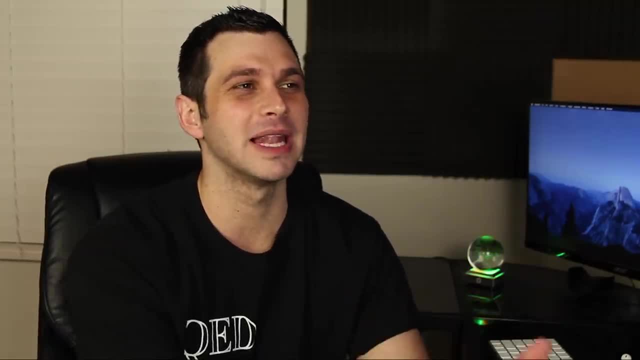 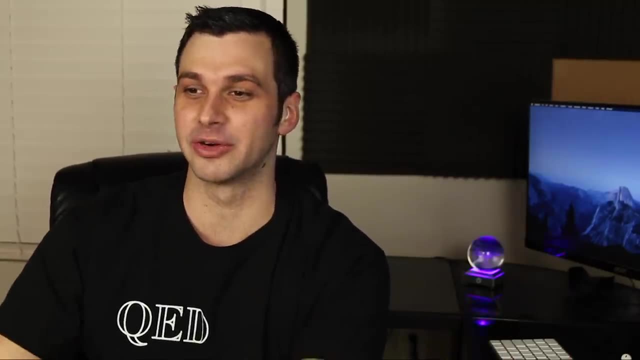 So learning this stuff rigorously. yes, it's not super applied directly, But you need that understanding to move on to the more advanced courses so you can rigorously define things That do have applications. Okay, now some other things I wanted to answer. 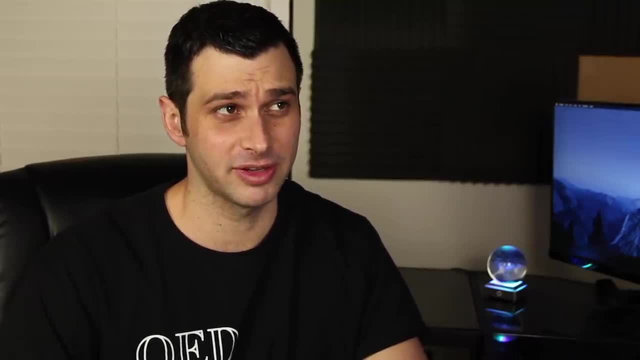 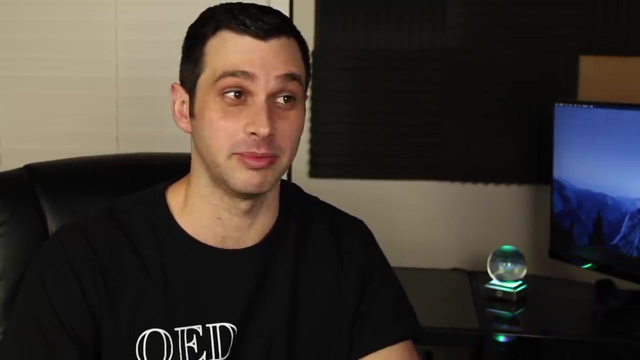 How long did it take me? About four and a half months, I want to say, And I worked on it not every day, but it was almost every day, And my breaks were no longer than one or two days. Sometimes I would just do it for like 30 minutes, which was often one practice problem, if that. 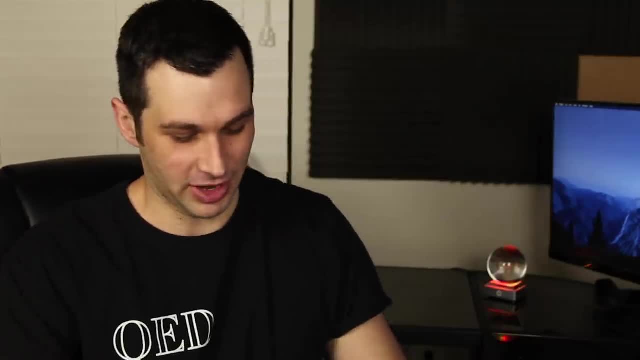 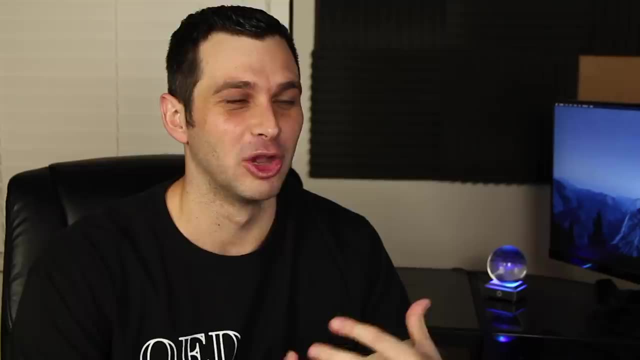 Or reading through a part of a section, But often it was, you know, I'd have to spend a few hours on it And I made videos based on some of the stuff I was reading, because it kind of helped me learn it better. 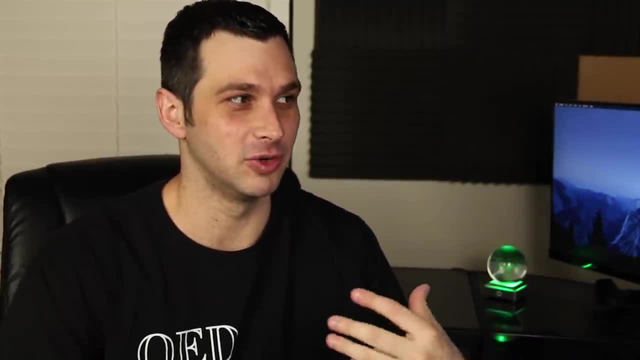 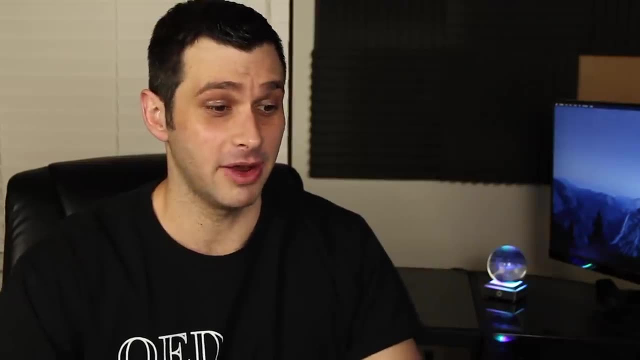 I had to really make sure I understood it. for the video It allowed me to, you know, review it again and, you know, get it more into my brain. Those were some of the infinity videos that I did, But yeah, no, I went through the entire book, every section. 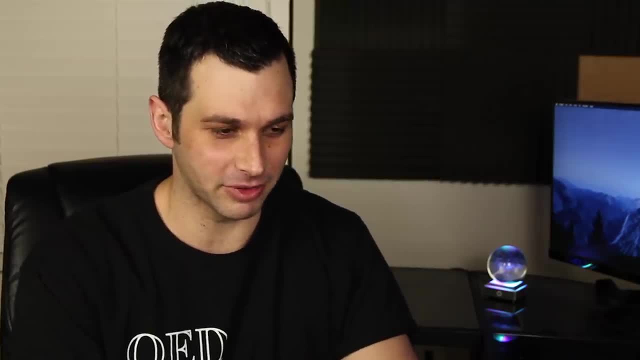 I did not do every practice. problem, And that's the one tough thing about self-teaching: You aren't sure when you can move on. When you're in school you're told: hey, do you know? one through 20.. 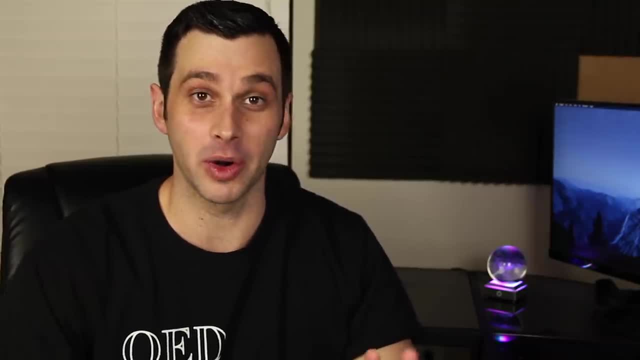 You're like: okay, I'm going to do this, I'm going to do this, I'm going to do 20 even. And then you know: okay, that's good enough, for my teacher would have given me more. If you have ten practice problems at the end of a chapter here, you don't know whether. 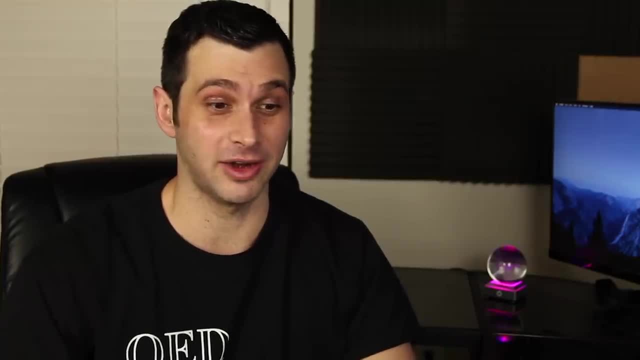 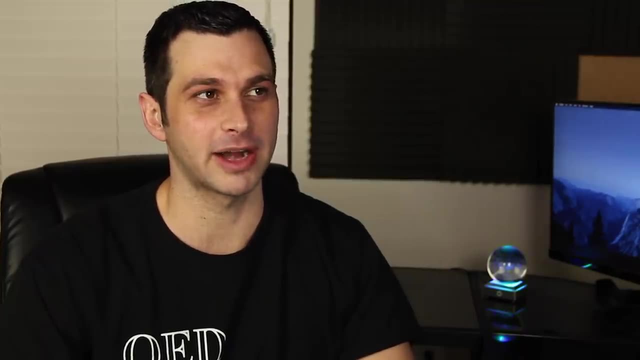 you could do five and move on, or whether you need to do all ten, or whatever. My general rule of thumb was, I had to do at least four. Four to five practice problems at the end of each section. There were usually no more than 12.. 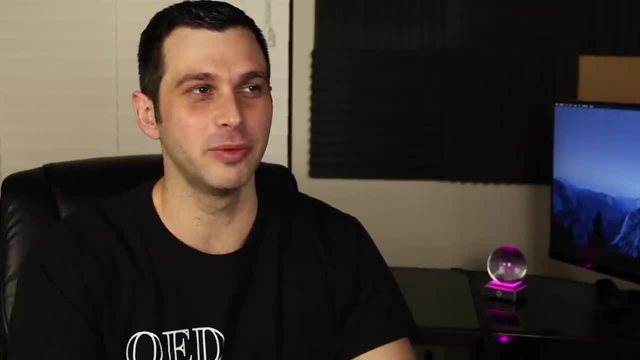 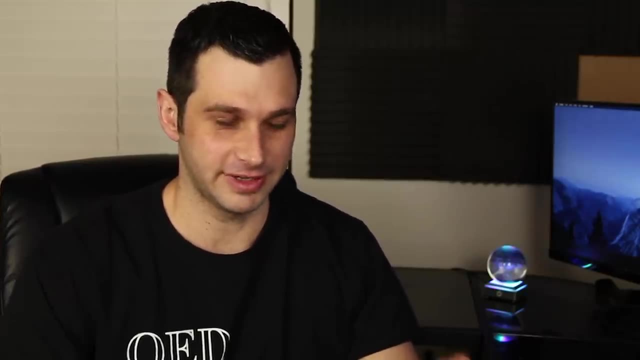 So about a third to a half of them for sure, And then I'd do more if they were, if they looked like Good problems that I should probably know. Something else important with teaching yourself a textbook is that you don't have anyone forcing. 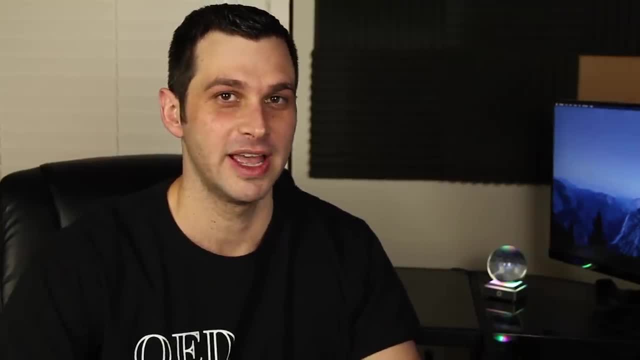 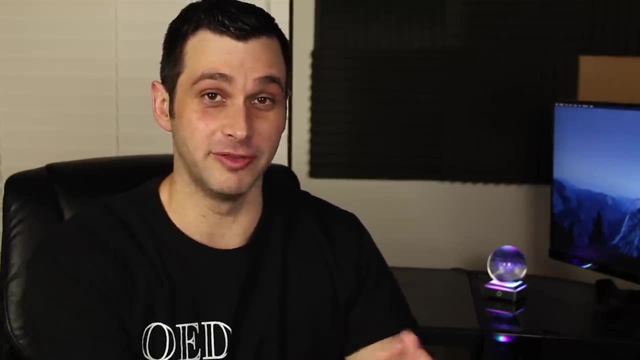 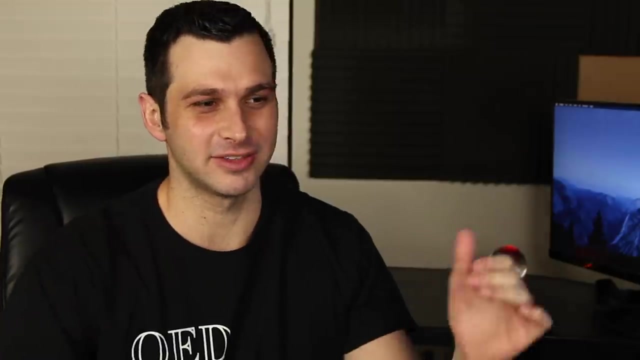 you to do quizzes and tests and review your knowledge And you'll find that actually is more important than you realize. The reason we take tests and all that it forces us to review that information or not, But most of you probably do. And when you do it again, all that, all that stuff you learned two, three weeks ago again, 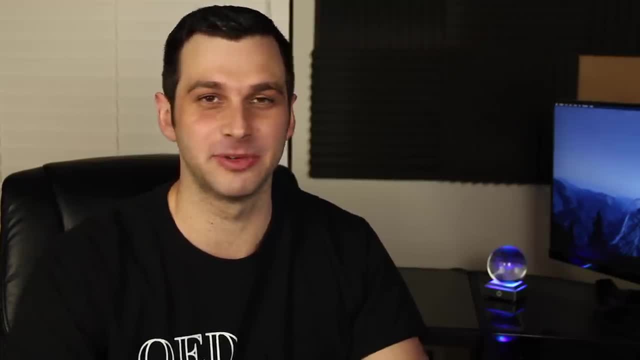 it gets into your brain much more. You remember it much better than you realize. There were often times I would just do the practice problems, move on, and I'd look back after like a week or two, realize, oh, I don't totally remember how to do this. 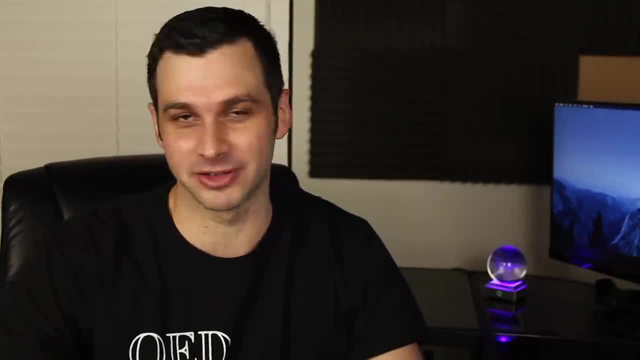 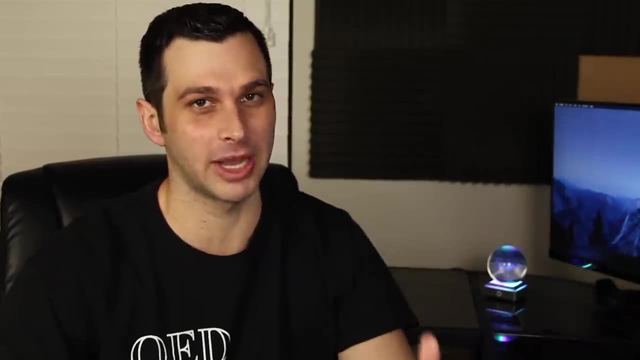 And when I do it again, then I could repeat it, you know, even after four or five weeks. So the things I remember now are the things I reviewed again or that just kept showing up in the textbook, so I really couldn't forget them. 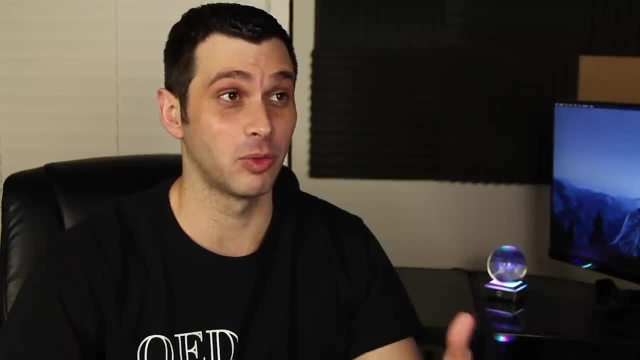 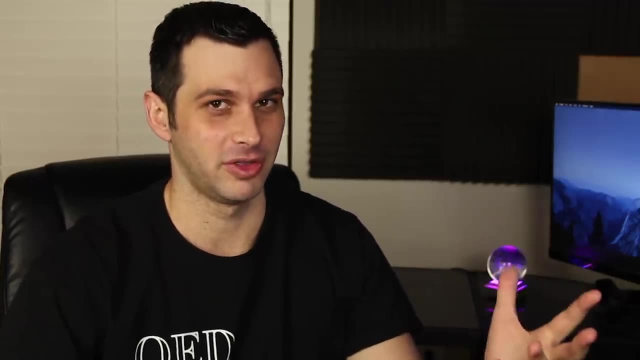 So that's something important. So if you're doing the practice problems, maybe skip over one or two and then, at the end of the chapter, go through those one or two that you skipped, because it will help you remember the information from that chapter better. 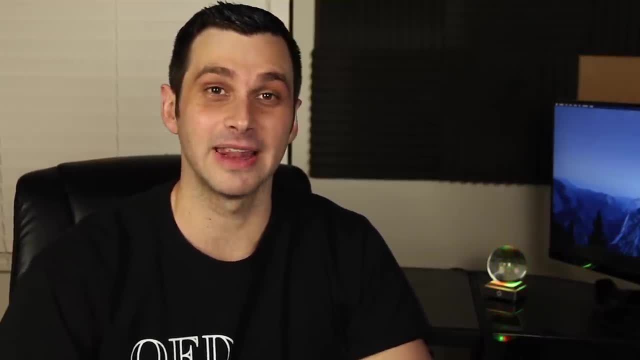 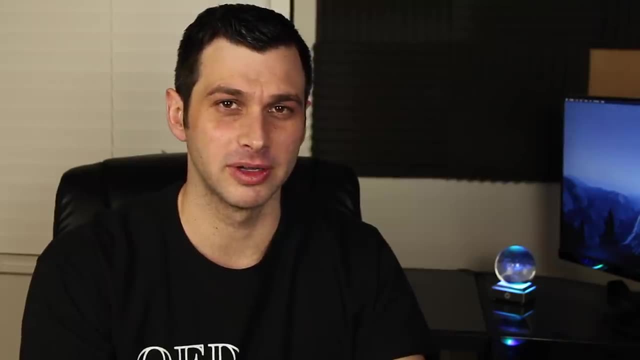 Just a general piece of advice. Something else I wanted to answer was: did I like this book much more than I thought I would? Because, as you can guess from my channel, I like applied math a little more. I guess I really hadn't done much pure math, but I like applications a lot. 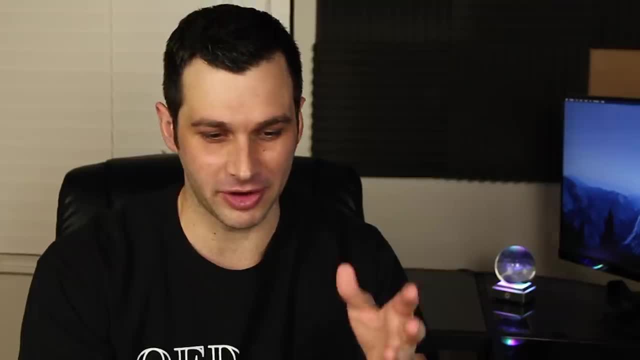 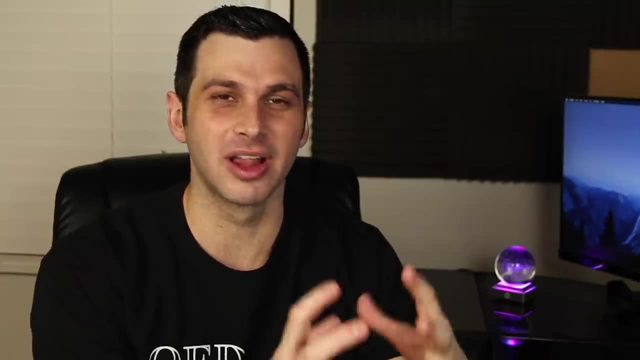 But often when I was going through these questions- whether I had to look at the answer or whether I was able to figure it out on my own- I liked the solutions. I thought they were clever often. This is not a book where you're given a formula, then you go apply that formula. 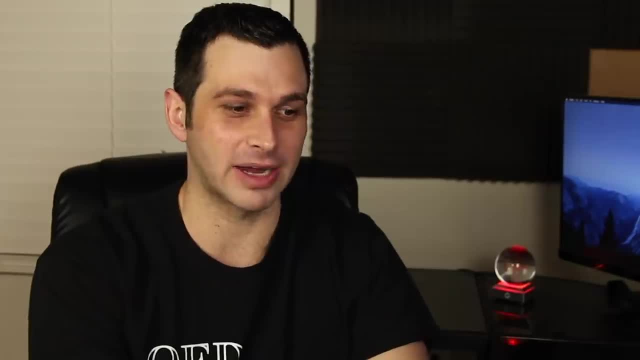 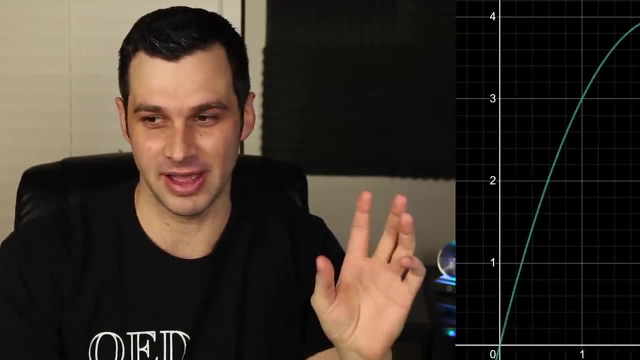 You have to think, You have to be creative, You have to think abstractly. in a lot of these cases, For example, you prove Rolle's Theorem, which is a Calc 1 concept. if you have a function where you have an a interval a to b and f of a is equal to f of b, then you know if 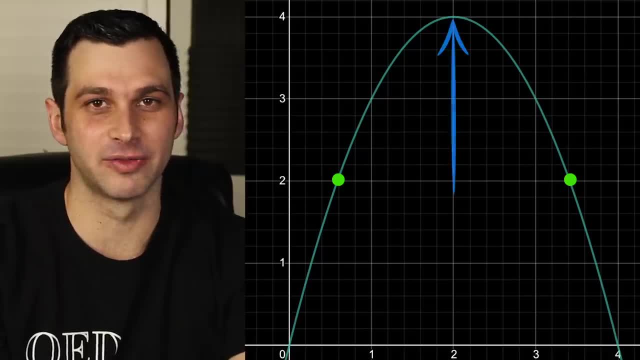 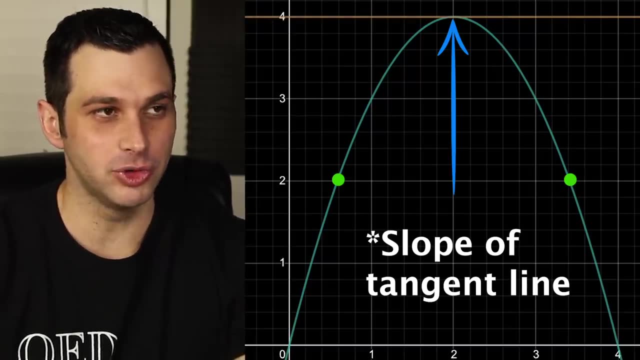 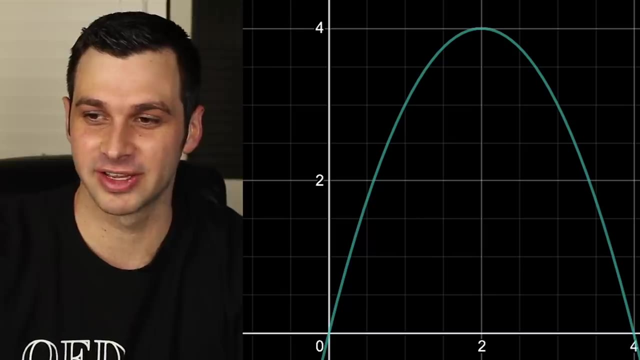 that function is differentiable, that you have a point in that interval where the tangent line, the derivative, is zero, And then they ask you later in that chapter to use that to prove the mean value theorem, which is where you have some differentiable function f of x and an interval a to b. 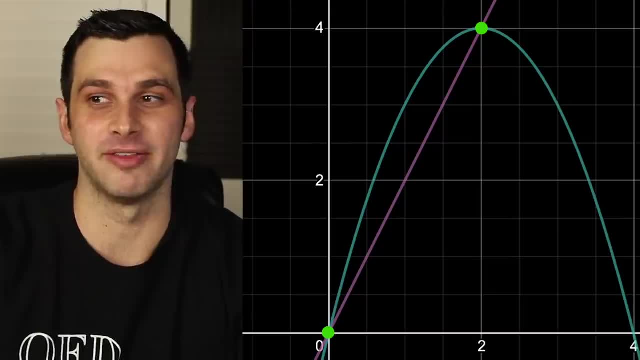 And you have a secant line going from the point a, comma f of a to b comma f of b that the mean value theorem says. there's a point in that interval where the derivative, the slope of the tangent line It, matches the slope of that secant line. 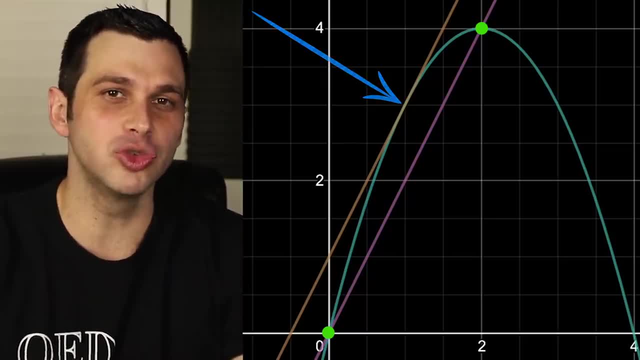 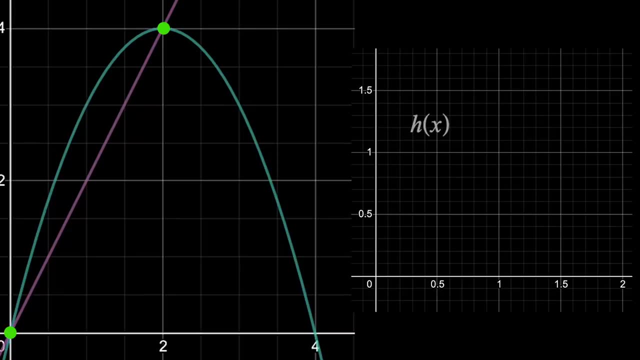 And you have to prove that's always true for differentiable function using Rolle's Theorem. The proof was: make a new function h of x. that is the difference between your function f of x and the secant line. I can call g of x. 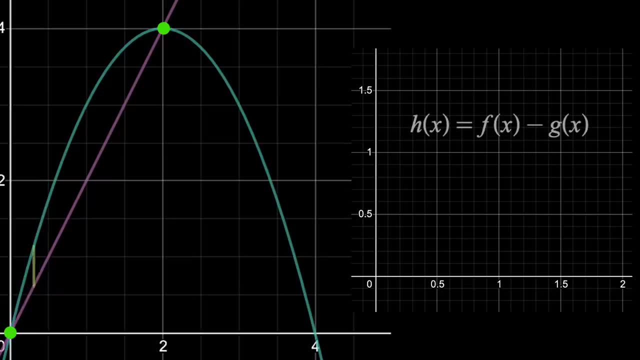 And that difference will be zero at the end points because the secant line intersects the function at those points. So on this interval h of x will start and end at the same y value. We sketch out the rest of the function by taking those differences. 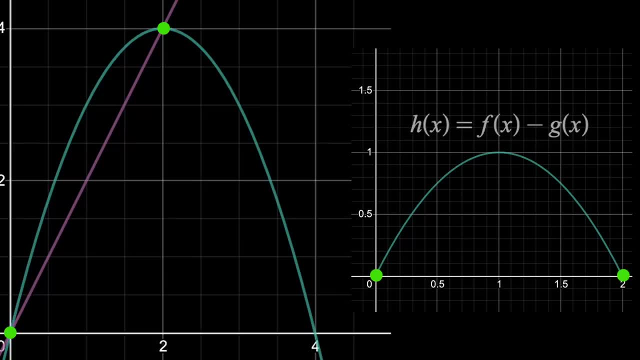 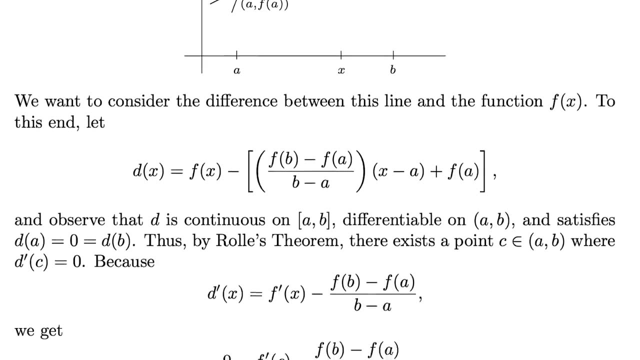 And now we can apply Rolle's Theorem to this because of those matching y coordinates And when you go through with Rolle's Theorem using the actual equations, the mean value theorem pops out. When I see stuff like that, I think that is. that's interesting. 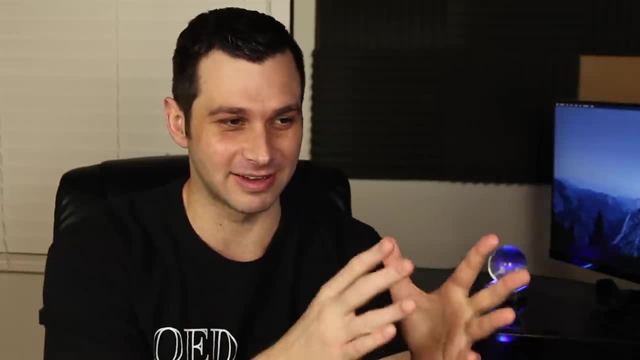 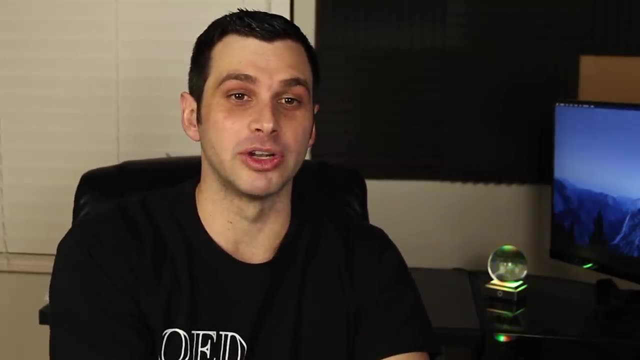 I would not have thought of that on my own, probably, but I like that. That is clever. It wasn't something you're just told to do, So you have to kind of think creatively. Okay, When you see that once you can use those techniques later. 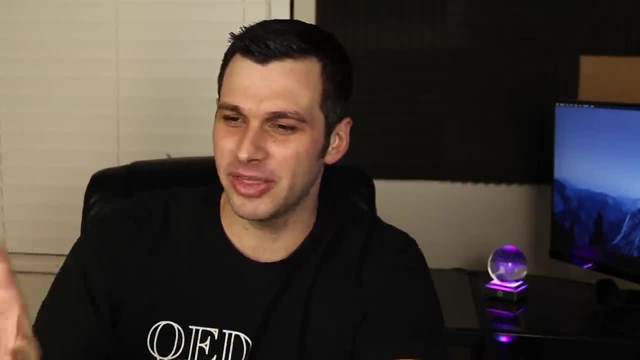 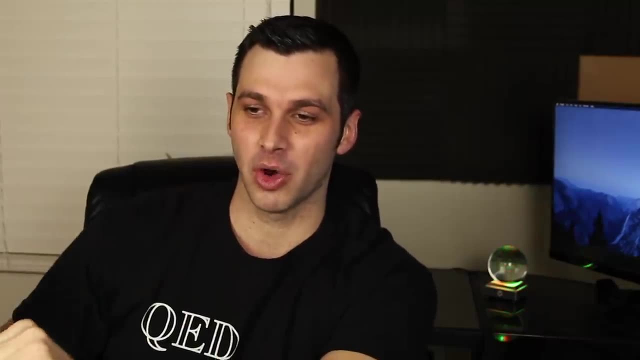 And that did come up- where you have this general f of x And you don't know anything about it. I don't know where it starts and where it ends, but I can use certain techniques to map that function to a new one where I have more control or more knowledge over the end. 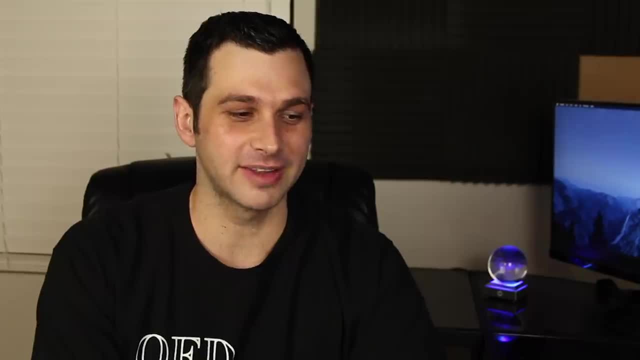 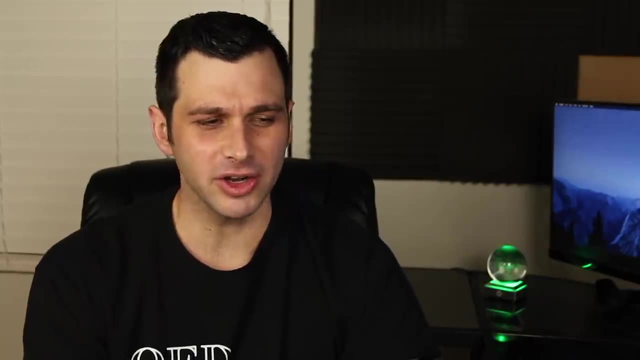 points or the y coordinates or whatever it may be. So that's the kind of stuff with this pure math class where you got to think more creatively. It's not like calculus or precalc. And then I talked a lot about strategies with self-teaching in the last video. 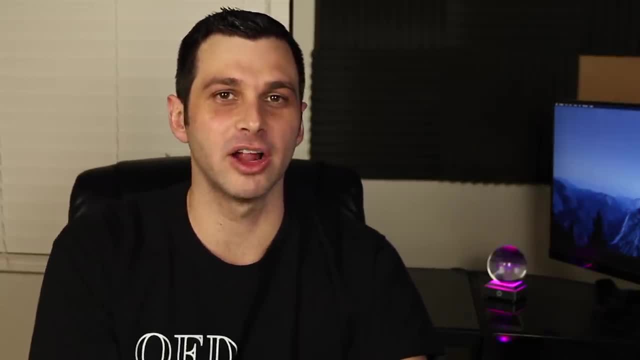 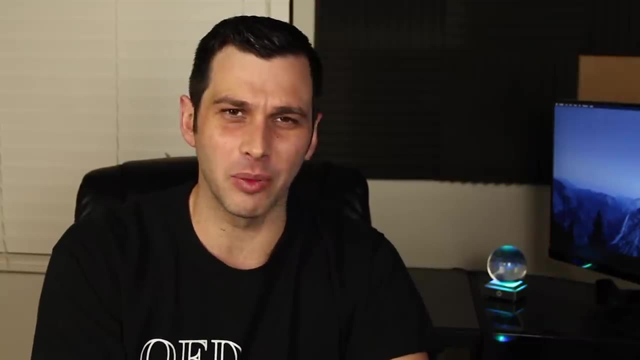 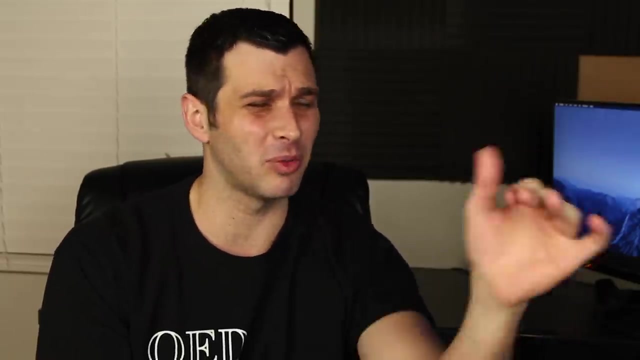 So check that out if you want some more of those. I will say one question I get a lot is people being discouraged by not being able to get through certain problems or when they get stuck on that one page where you have to read that paragraph eight times and you start to kind of you're like, okay, I sort of get. 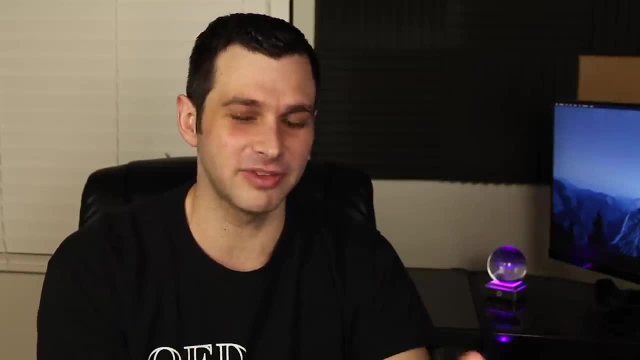 it. but why is this like that? You just it's tough to get through. People get discouraged by that a lot. Let me just say this: That will always happen. If you go to self-teach yourself, if you go to teach yourself something new, you are going. 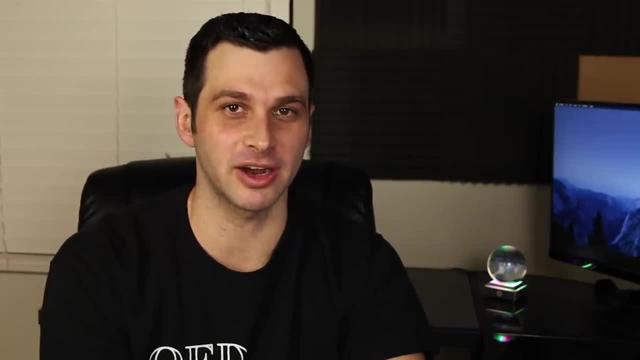 to hit a point, most likely where you are genuinely stuck. okay, It's not about trying to avoid that. It's as you teach yourself: more you learn to fear, that less You won't be scared when that happens, because you'll know- oh, I've been here before. 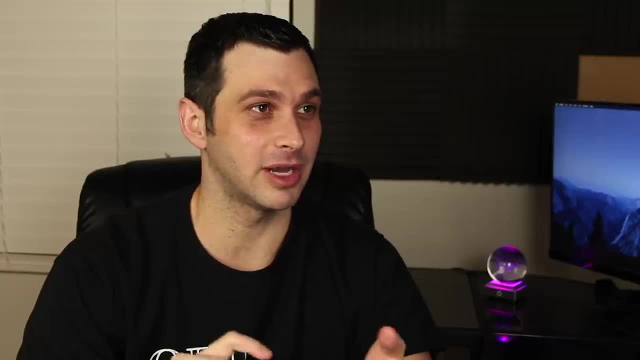 I'm either going to read this over and over, I'm going to look up YouTube videos, I'm going to go on some forums. I'm going to go on some forums to figure it out. I will figure it out And you just start to fear that less and less. 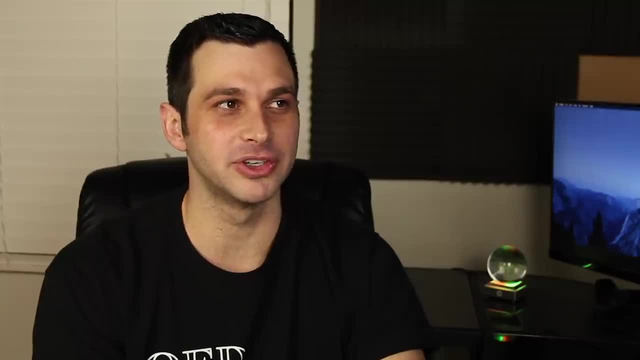 So that's something to keep in mind. You're going to hit a point where you're just stuck. It happened to me, like every section of this book, honestly, where you just start reading and then you'd be like what, how'd you get to that? 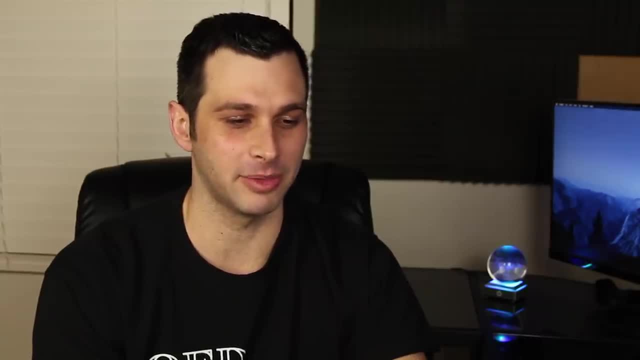 They use the word obviously way too loosely in upper level math. I'm starting to realize, oh, this is obviously true. I'm like what? No, it's not. And then I figured out like 10 minutes later I'm like, oh yeah, that was obvious. 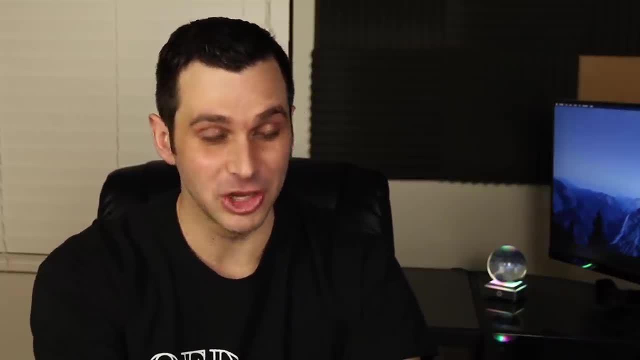 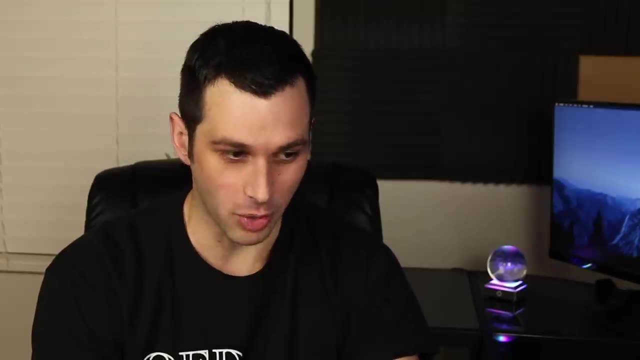 Once you realize it. but yeah, sometimes you are just stuck like that, So realize it's not just you, It's me too And it's pretty much everyone around you. And going through a textbook is slow. You can spend an hour reading a page. 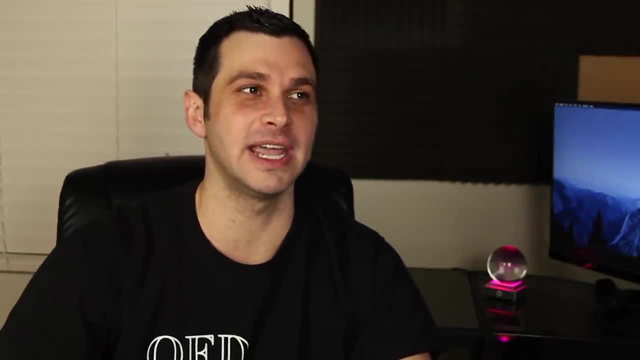 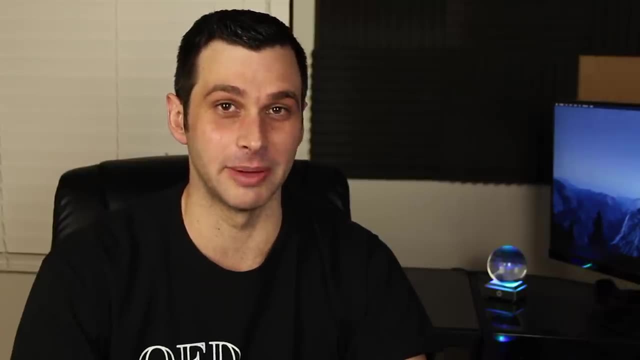 That is fine, That is normal. Sometimes you have to do that, especially in a pure rigorous class like this, And I'm sure the same thing would be true for many upper level STEM courses. Oh then, regarding practice problems, When you also are genuinely stuck. 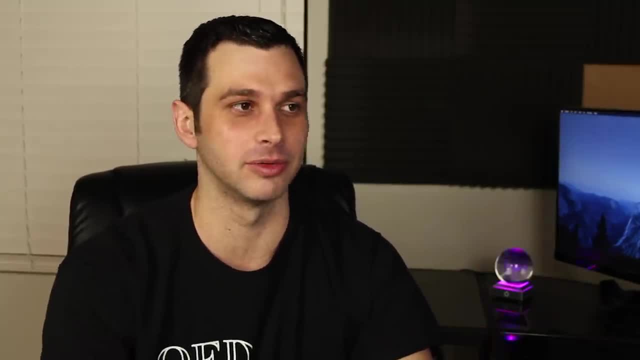 And you can't figure it out. when you want to give up- which I had, I did- do So. don't freak out. if you have to give up on a problem, Don't feel defeated. Here's what I did when that happened. 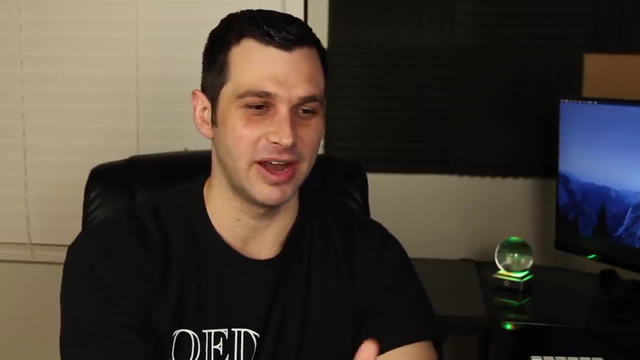 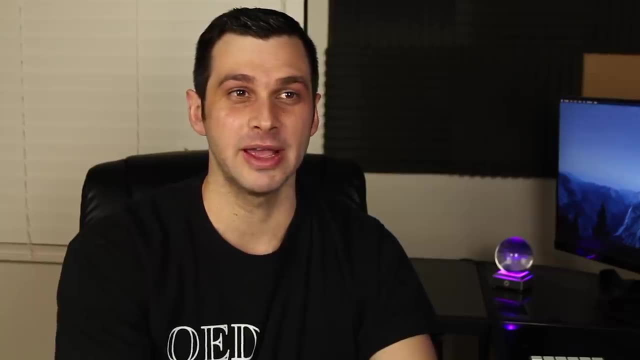 One: make sure you have a textbook- I recommend it- that has a solution manual, or you can find it online, because there were times where I was like: oh, I know how to do this problem And I went through it and I almost just moved on because I knew I was correct. 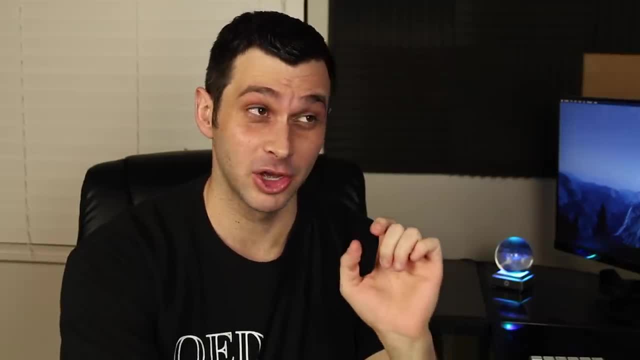 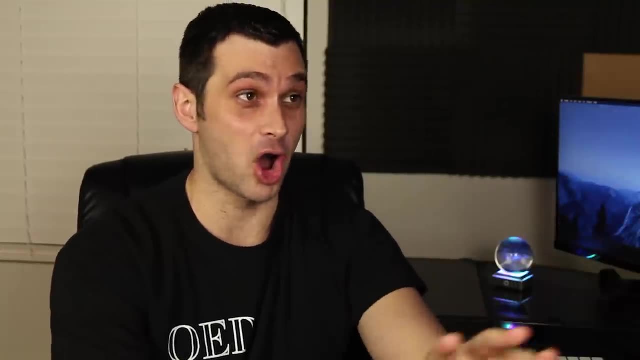 And then I look up the answer and realize there was something subtle I missed, And sometimes the book even knew that They're like: if you did this, Which is what I did, You're wrong. It's a common mistake students make. 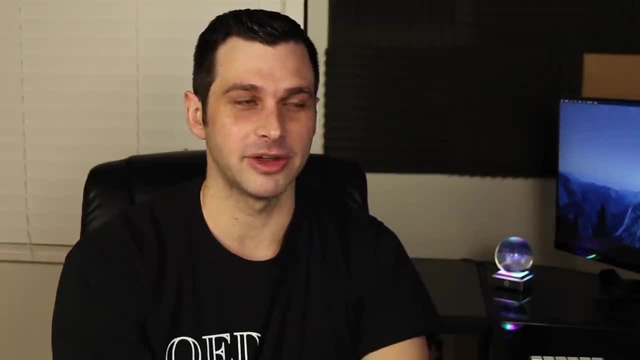 So that's why I recommend having the solutions. If you have to look up the answer, look it up and understand first why that is the answer. Understand why the solution is what it is, Because if you just look and say, oh okay, whatever. 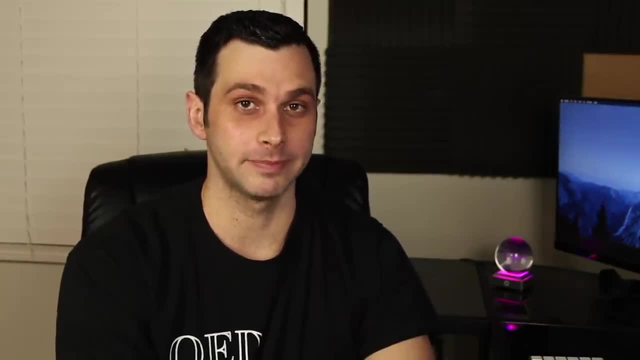 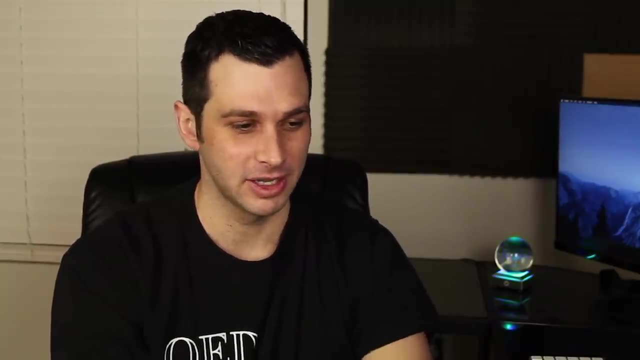 And then move on. you haven't learned it yet, So make sure you understand why Then do that problem again later, in an hour or a day, whatever it may be. Let your brain forget about it a bit though, because you'll find in an hour or a day, or 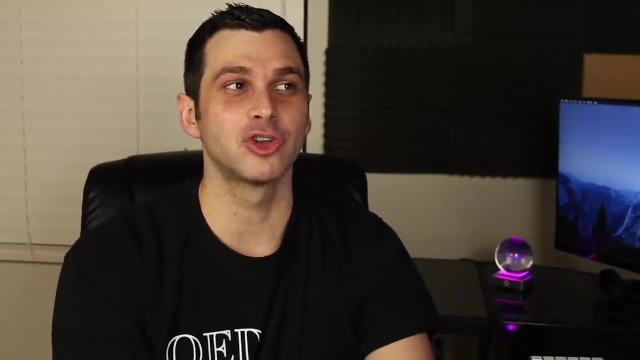 whatever that you might now again not totally remember, But it's kind of back to you're like: oh yeah, what did they have you do? It was first you had to do this And you kind of start to connect the pieces. 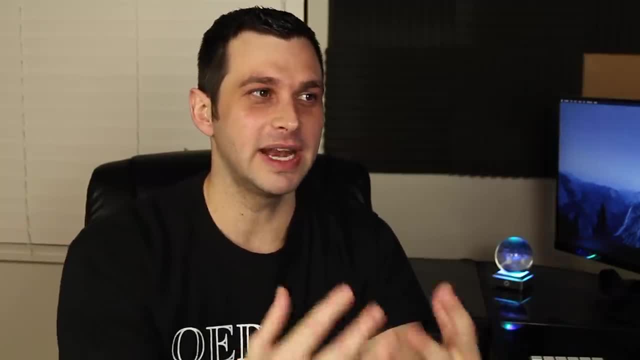 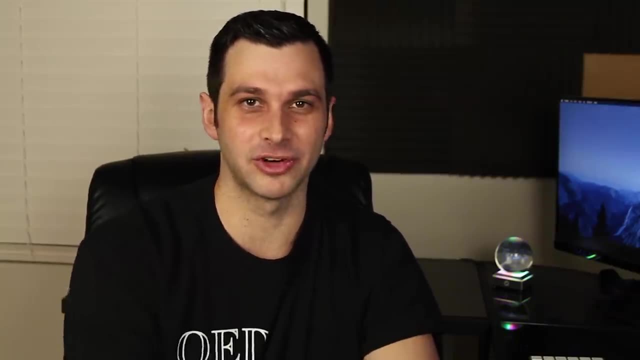 And once you do it on your own, it's in your brain. You did get it, As if you figured it out on your own the first time. in a way, You have the. you know why the answer is what it is. You know the techniques. 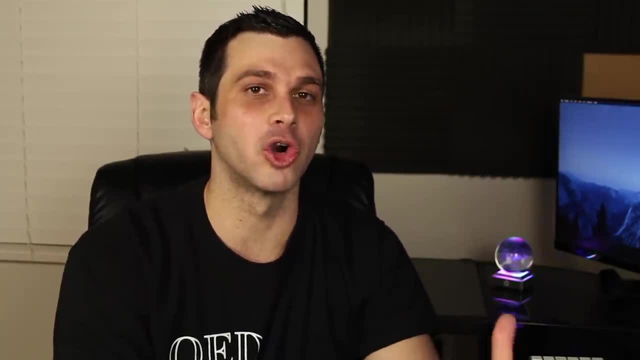 You know how to go from step one to step two. You did learn that question, even if you didn't figure it out the first time on your own. So don't freak out if you have to look at the answer I had multiple times in this book. it was so discouraging, honestly. 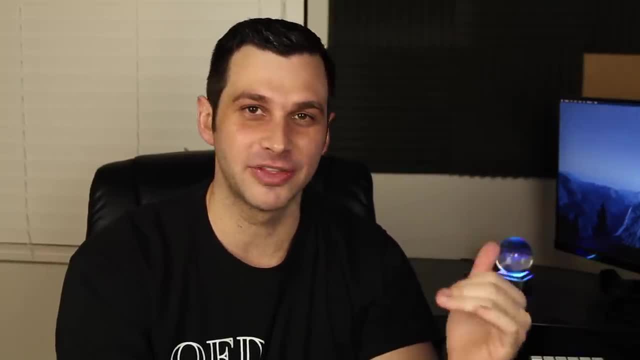 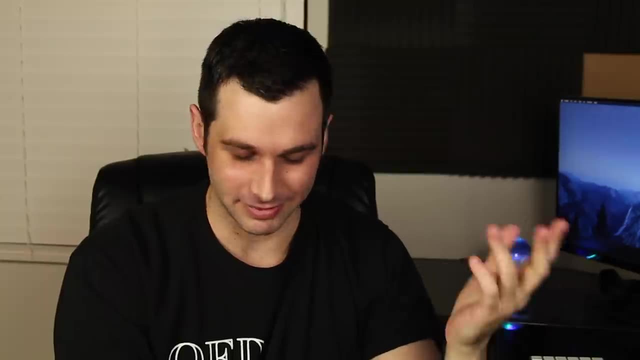 But it's okay. Where I'd do, I'd be on like question two. I'd sit there for an hour or two hours. After two hours I typically have to look it up, But I'd do in number two and I'd look up the answer and sometimes it was sometimes it. 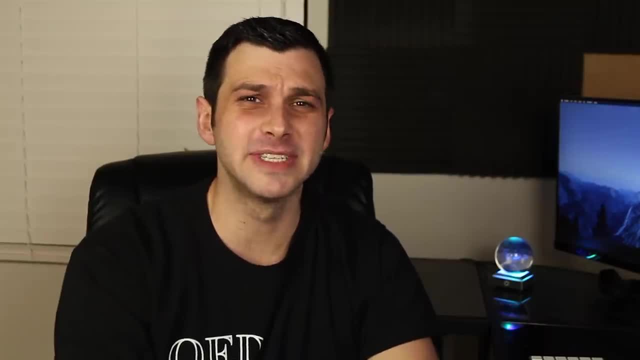 was real tricky- Like I don't know if I would have thought of that on my own- And sometimes it was easy. Sometimes I was like: why did I not think of that? But in my head all these problems were tough. 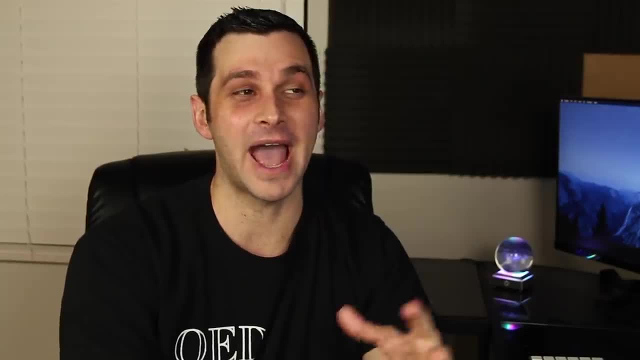 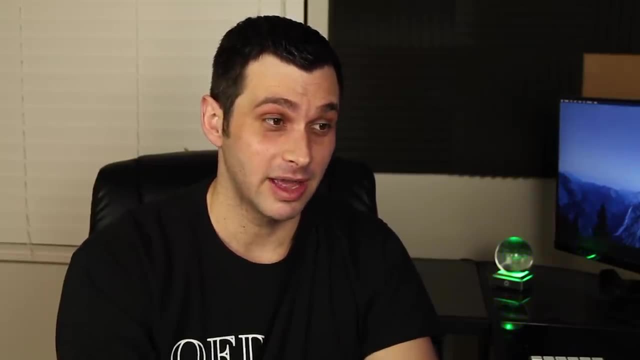 So I was always looking for something clever when I didn't really have to. So I was like crap, okay, missed that, Let's go on to number three. Same exact thing would happen. And then I'd move on to number four, and the same thing would happen. 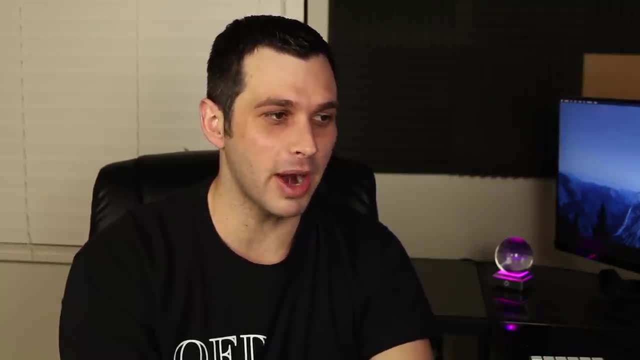 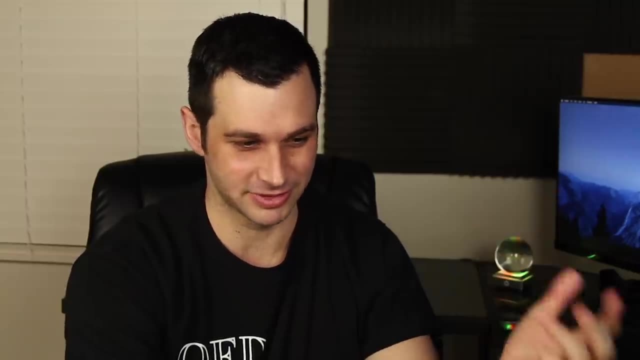 Sometimes it happened three or four times in a row. I was like, give me a break, Give me one I can solve. But that's the reality of a upper level Okay Level math, science, engineering based course. that can happen. 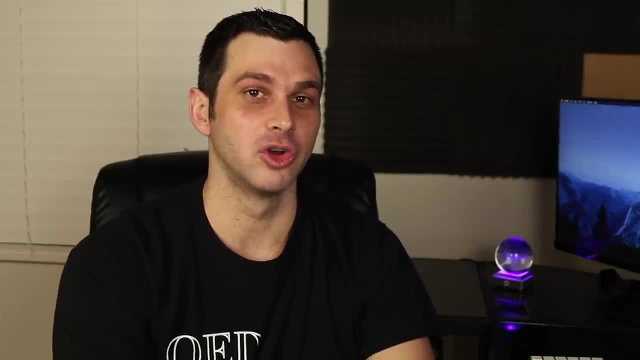 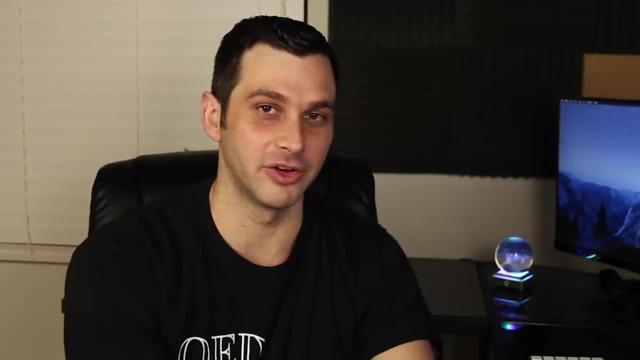 So just realize that and it's okay. But again try the problem again on your own later. Make sure you understand the solution, because if you just move on and give up, then you really haven't learned it. Oh, and that's something else I wanted to say. 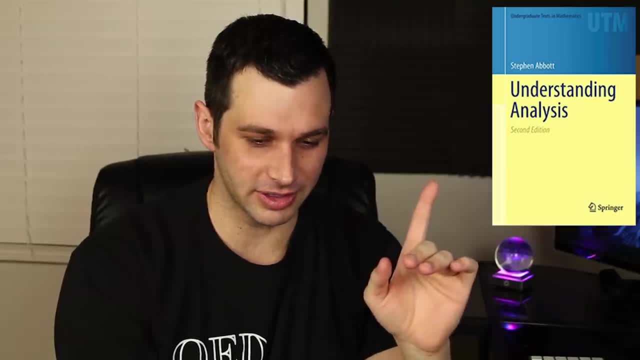 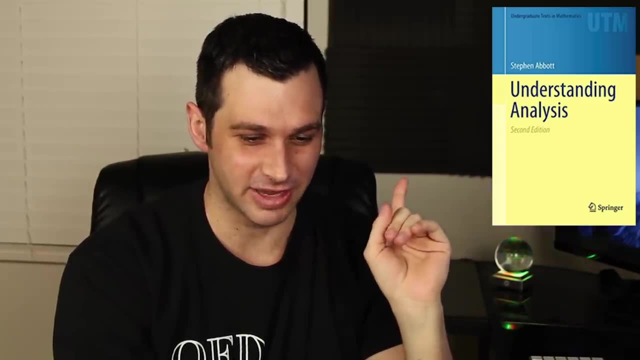 This is the textbook I used. This is, if you are going to teach yourself real analysis to this book. don't even think. just go with this book. It is the best real analysis book for self-teaching, in my opinion, just by going through kind. 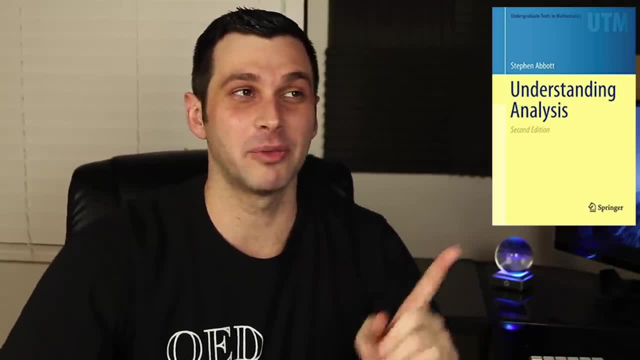 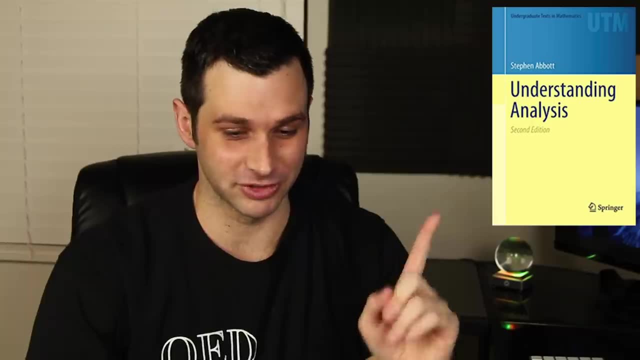 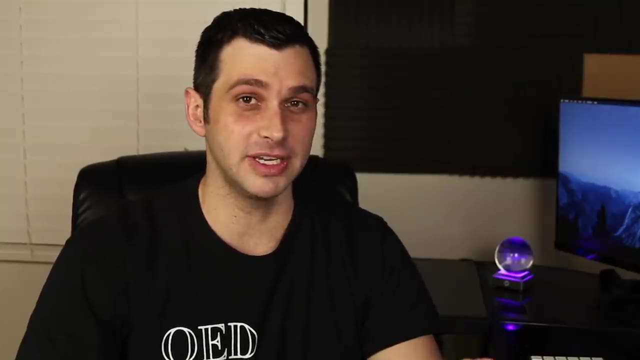 of a scan of other textbooks. This is not the main one they use in school. I think that'd be Rudin, I think that's what it was, But for self-teaching- this one. A lot of the times when I look up textbooks I want to use for self-teaching. it can be. 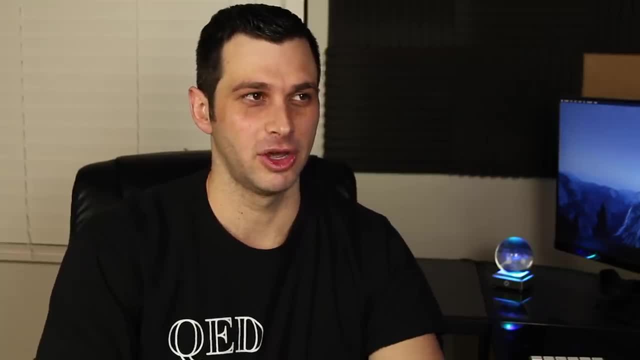 kind of tricky Because again, you aren't sure. Should I go with the most difficult and most real? No, Should I go with the most rigorous? Should I go for the easier book? Or will the easier book not allow me to move on? 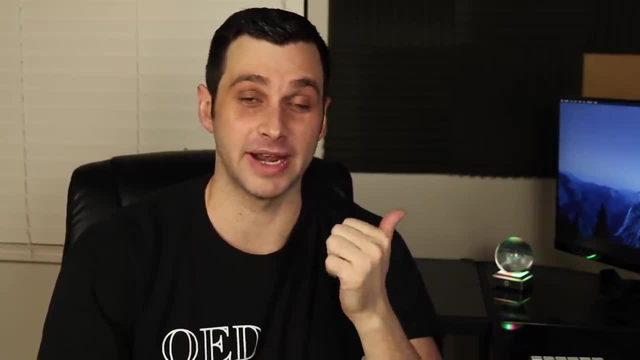 If you're self-teaching, you're probably in one of three categories. You're either doing it for the next semester or quarter of school, just trying to get ahead. You're to the hobbyist who's just learning it because you like this kind of stuff. 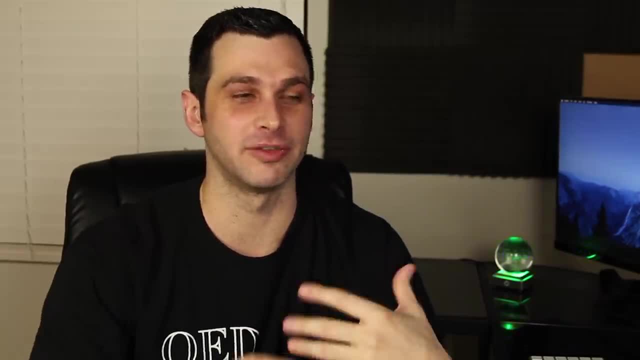 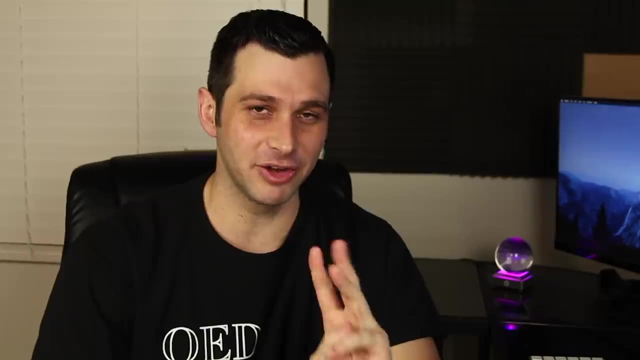 Or you're learning it for your professional life. You want to start a business, You want to make a product, You want to publish a paper off this kind of stuff. If you're in the third category, then you want to go for professional. 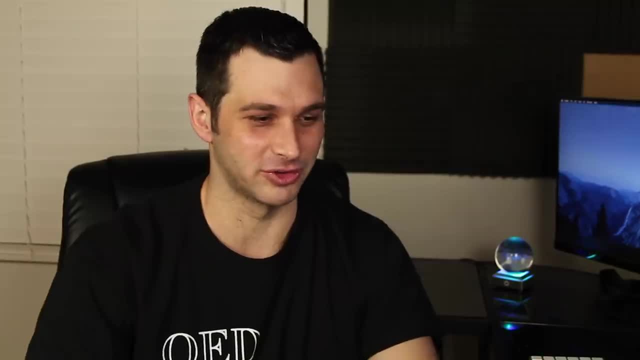 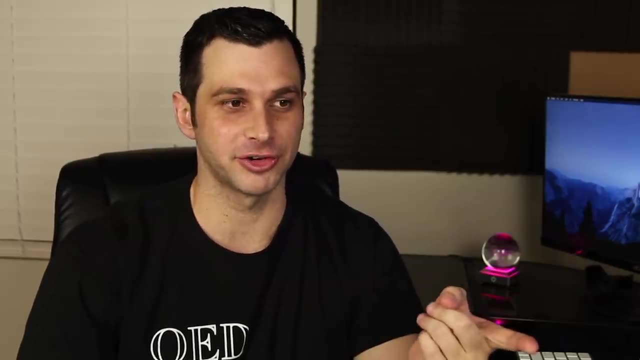 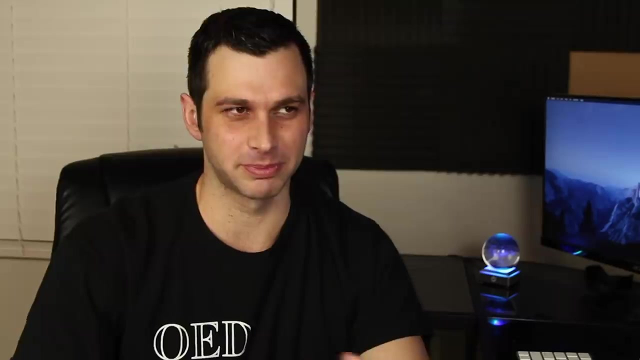 You're probably the most rigorous textbooks or courses or the ones that will give you the tools you need to achieve whatever goals you have. But if you're in the first one for school, probably get the textbook your teachers recommend you get. But if you're the hobbyist, if you're number two, which pretty much I am at the moment, 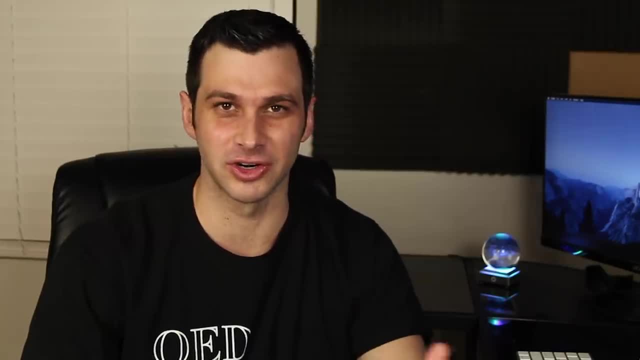 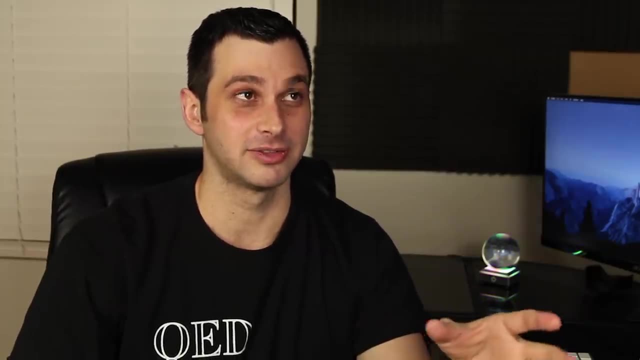 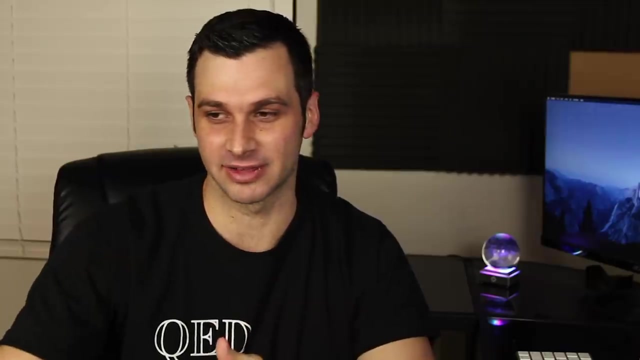 don't necessarily get the hardest textbook if it's going to discourage you especially. You know your level. But, for example, this book was slightly easier I read than some of the others, But it was still rigorous, It was very challenging And it gave me everything I need to move on to the next class. 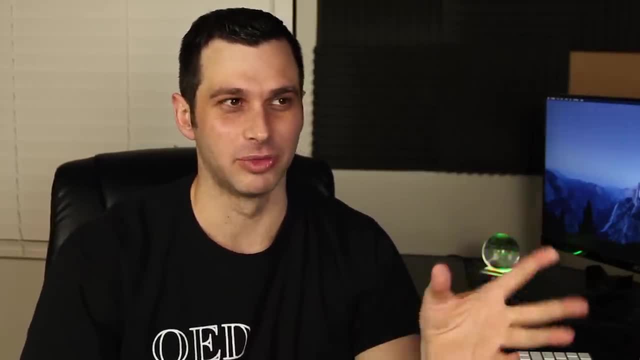 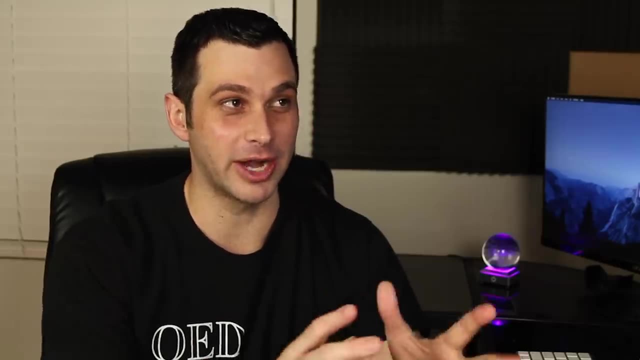 I'm going through a point: set topology book right now as well, And real analysis, I would say, is the prereq for that. Got everything. I need Everything. all the rigor that I need for the topology book was there in real analysis. 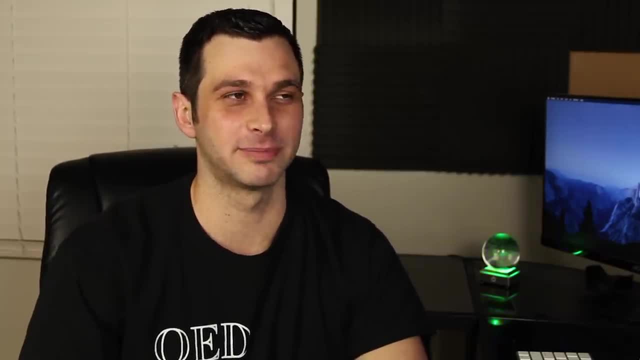 So don't freak out. if you don't get the hardest textbook, It's probably not going to prevent you from being able to get the textbook. It's probably not going to prevent you from being able to get the textbook. It's probably not going to prevent you from being able to get the textbook. 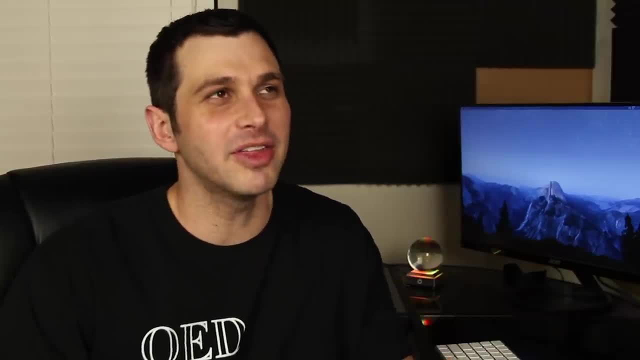 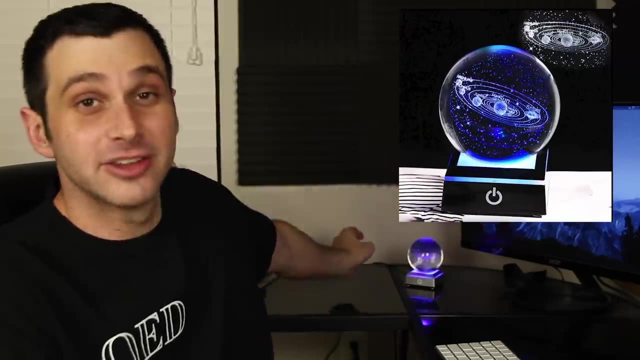 It's probably not going to prevent you from being able to move on. if that's what you want to do, All right. I think that's just about everything I wanted to talk about Real quick, if you want to get this LED solar system- you've seen changing colors here. 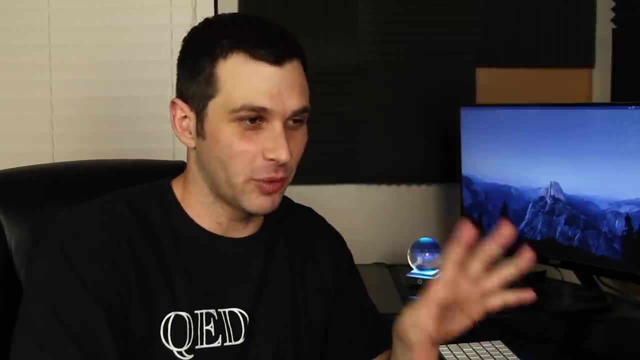 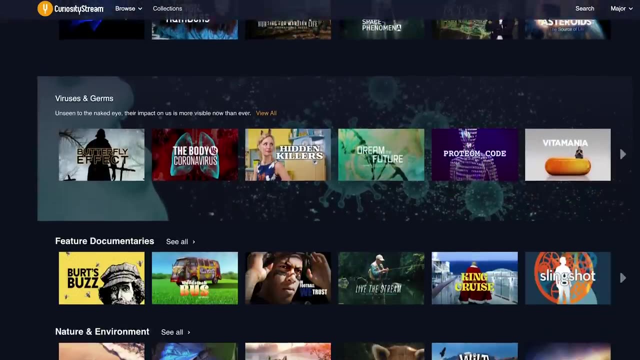 it is available on stem merch. Look out for the next video where I'll be showing you what one of these proofs looks like. And then, before we go, I want to thank CuriosityStream for sponsoring this video Now. even though this was a video on pure math, like I said earlier, I'm still a huge fan. 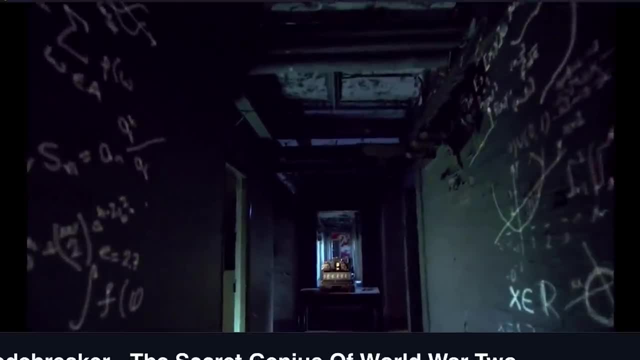 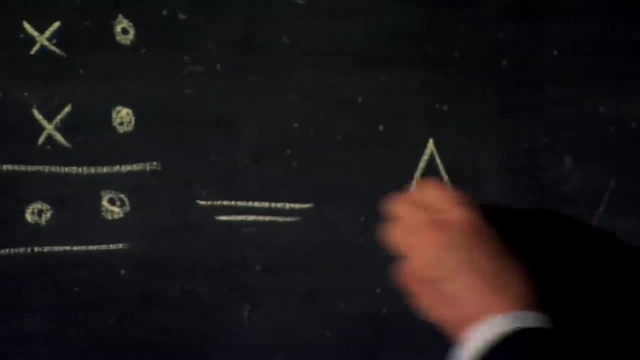 of the applied stuff. So one of my favorite documentaries they have on this platform is Code Breaker. This is the story of how mathematics and cryptography were used to help put an end to the second world war. However, this goes beyond Alan Turing, whose name is the most famous when it comes to this.